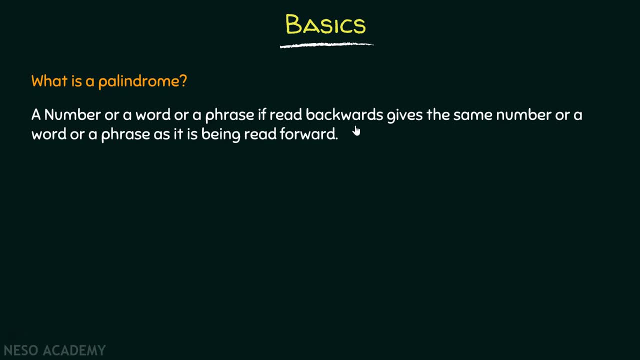 If we read it from the backwards, it actually gives the same result as if we read it from the forward. Let's consider one example Here. in this example, as you can see, this number is 1221.. If we read this number from the backwards, 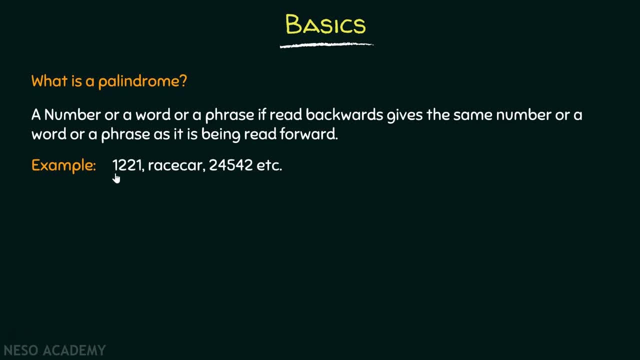 we can see this number is 1221, which is equivalent to the number that we read it from the forward. Now consider this particular word: race car. If you read this from the backwards, we can see that from backwards as well. 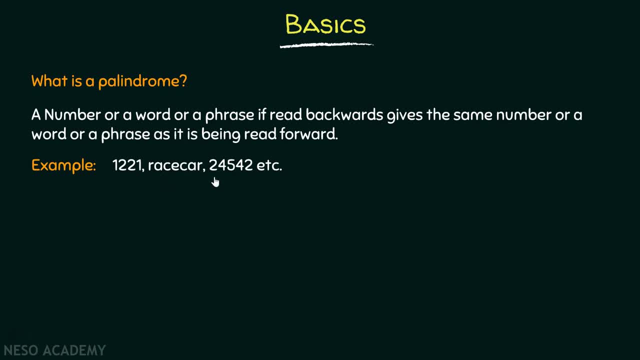 this is race car only, Right. Let me read this number now: This is 24542.. If we read it from the backwards again, this is 24542.. Therefore, this is also a palindrome. Okay, Now the question is: 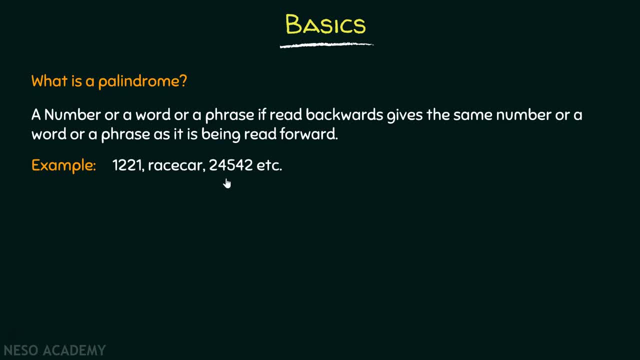 what idea we need to adopt in our program so that we would be able to give this answer, whether a particular number is palindrome or not. Here in this presentation, we will consider the program which tells whether a number is palindrome or not. We will not consider the strings here. 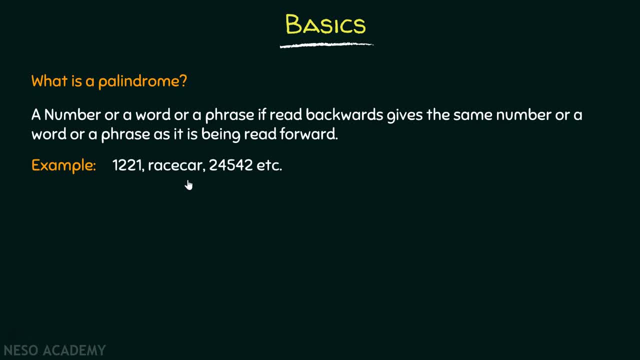 We will only consider the numbers. Now, what idea we need to adopt? The basic idea is make last number the first number, second last number the second number, and so on. What does it really mean? It simply means that you need to reverse the number. 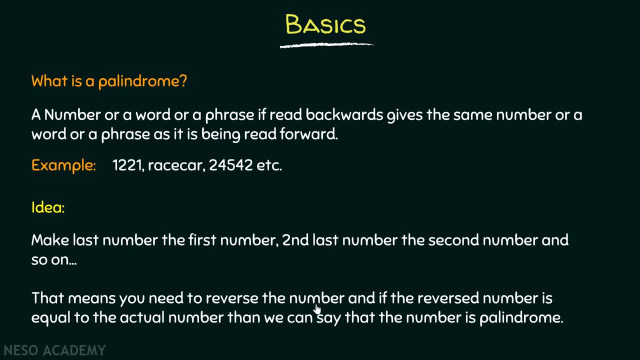 Please note down. you simply need to reverse the number, and if the reverse number is equal to the actual number, then we can say that the number is palindrome. This simple idea we need to adopt in our program as well. Now, our central idea is: 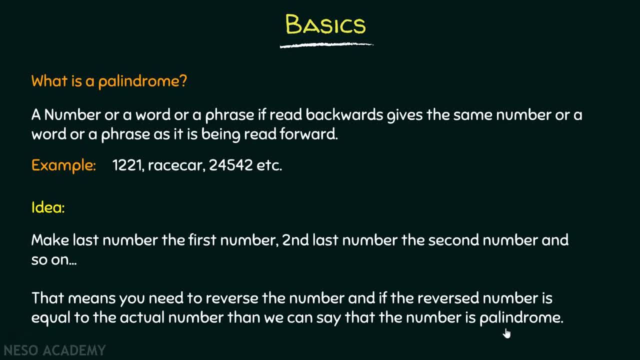 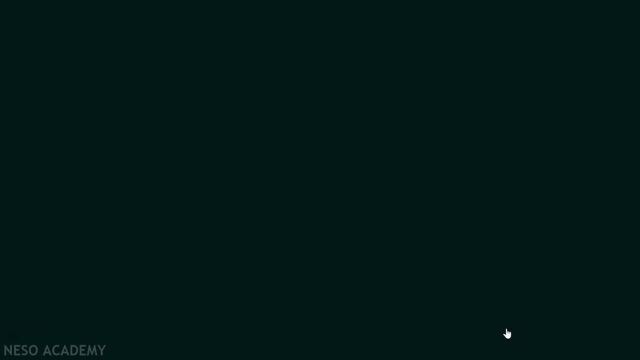 to reverse the number. If we would be able to obtain the reverse number, the rest of the part is easy. Right, We would be able to obtain the reversed number. Now let me ask you one question: What happens when we divide the number by ten? 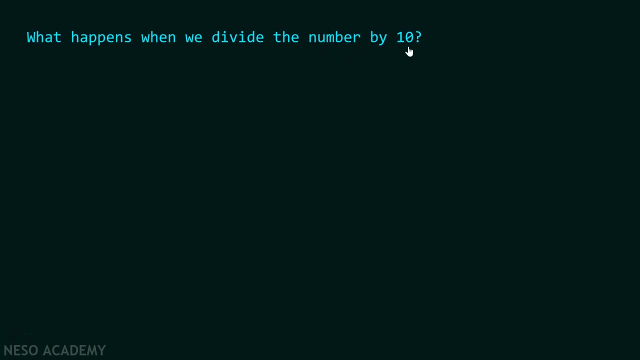 Suppose we have some number and if we divide that number by ten, what will happen? I will tell you one important property: When we divide any number by ten, then the remainder that we get is always the last digit of that number And the quotient that we get. 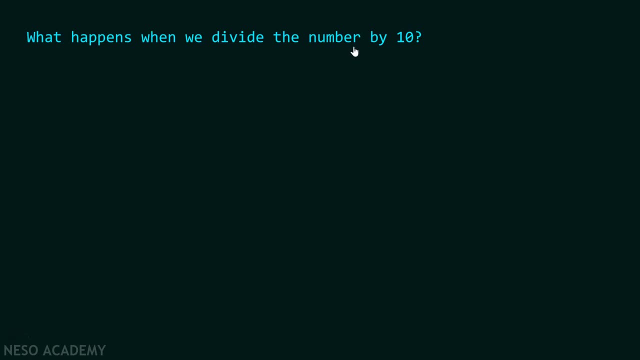 is always the number, except the last digit, Like, for example: if we divide 456 by ten, the remainder that we get is six, which is the last digit of this number, And the quotient that we get is 45,, which is the number. 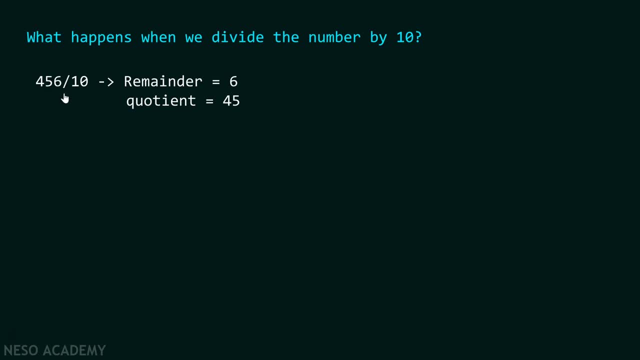 except the last digit. By using this property, we would be able to reverse the number very easily. How can we do that? Let's suppose we have a number 2332.. If we divide this number by ten, the remainder that we get is two. 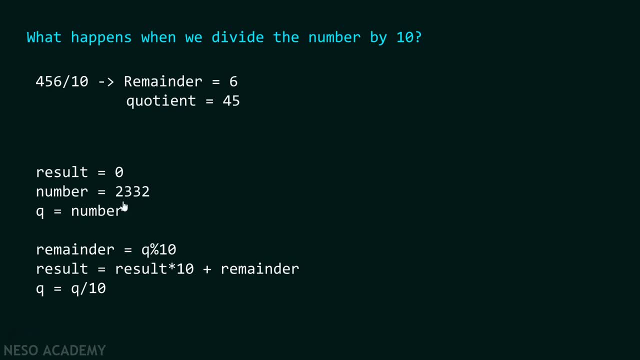 and the quotient that we get is 233.. Right, So initially we divide this number by ten and we store the remainder inside the remainder variable. Always remember that mod operator is used to find out the remainder of any number. Now, this is the logic we need to understand. 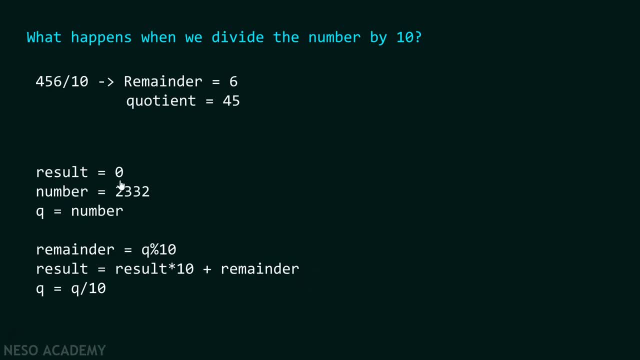 very carefully. Initially we are letting result is zero. We simply multiply result by ten and add remainder to it. This logic helps us to reverse the number. After that we have q equals to q divided by ten. q is nothing but denoting the quotient. 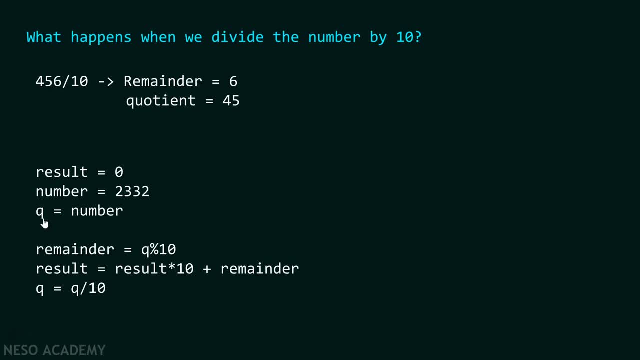 We are initially storing number inside q and then after that we simply divide this number by ten. Initially, the value inside remainder is two Right, As when 2332 is divided by ten, the remainder would be two only. After that we multiply result by ten and. 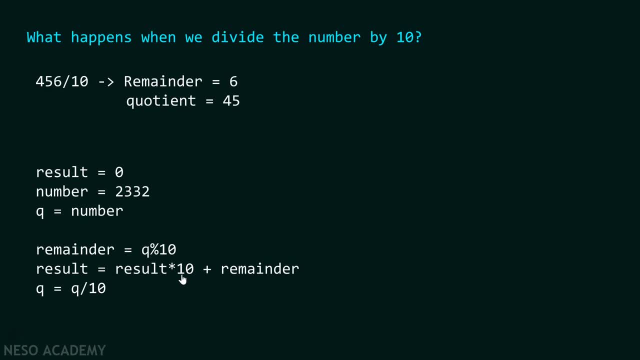 add remainder to it. If result is zero, therefore, zero will be added with remainder, that is two, and it will be stored inside this result variable. After that, we simply divide q by ten. Therefore, q will now contain value 233.. Now, what is the next step? 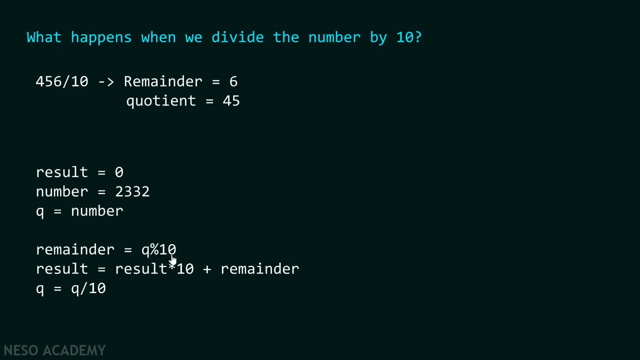 We again divide q by ten and store the remainder As q is 233,, therefore remainder variable will contain three. Right Next step: we simply multiply result by ten and add remainder to it. As result variable contains two, we multiply two by ten. 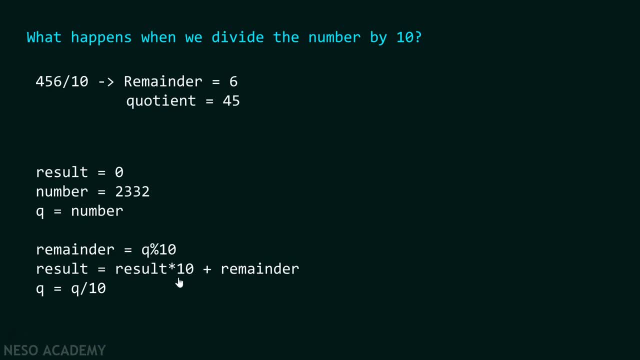 and add three to it. Now the result contains 23.. Now what is the logic behind that? If we multiply two by ten and add three to it, we would be able to reverse this number. Previously, the number is 32.. If we want to reverse this number, 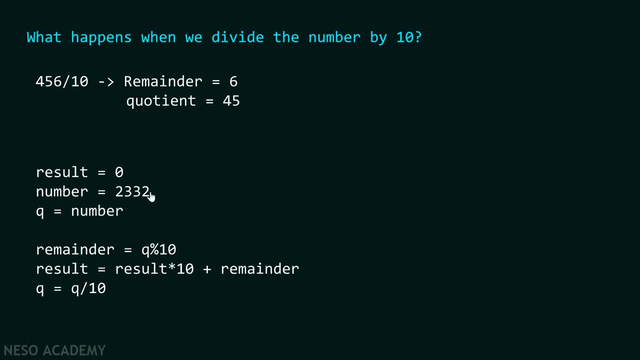 that is, if we want to make this number 23,, we need to multiply two by ten and add three to it. This logic makes it 23.. And that is what we are doing here Now. the result variable contains 23.. After that, we simply divide. 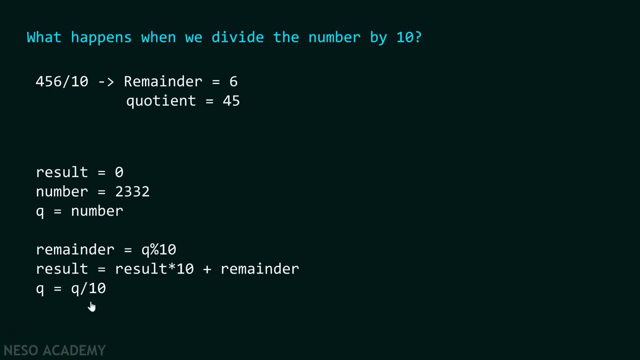 q by ten. After dividing q by ten, now q contains 23.. Then again we repeat the process. We divide 23 by ten and store the remainder. Now the remainder contains three. and then what we do? We again multiply, result by ten. 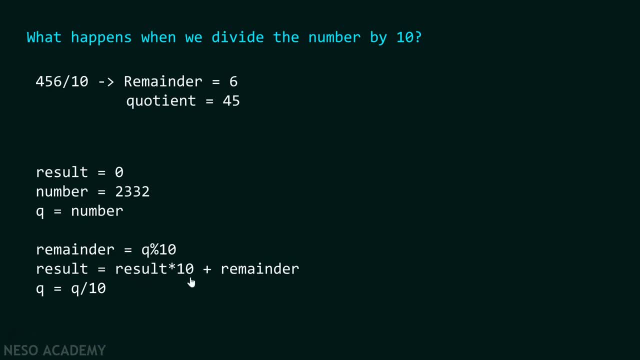 That is 23 by ten, That becomes 230.. We add remainder to it, That is three. Now it becomes 233, which is the reverse of 332.. Again, we repeat the same process and finally we would be able to obtain the reverse of this number. 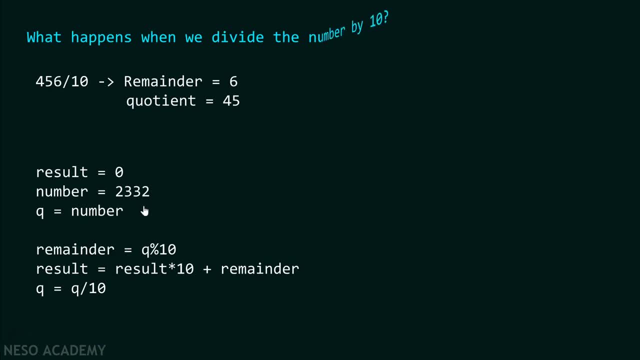 This is the logic we need to understand Now, definitely. the final step is to check whether the result is equal to the actual number or not. And if it is equal to the actual number, then the number is palindrome. Otherwise, it is not a palindrome. 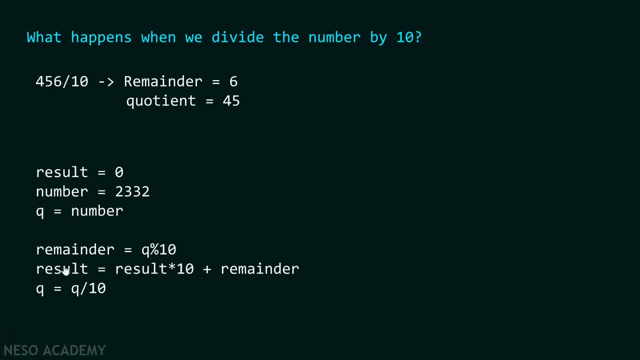 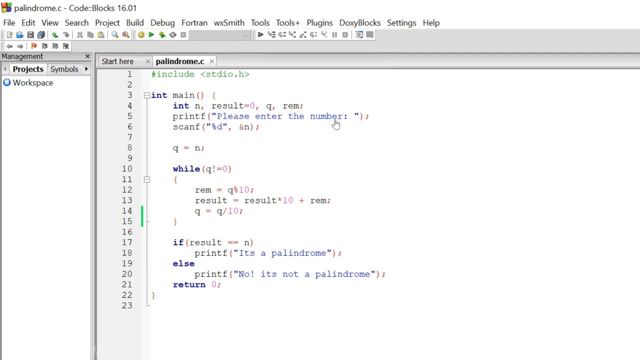 Now let's see how to code this particular logic. Here you can see I have one printf function and inside this printf function I am printing: please enter the number. That means I am asking the user to please enter the number. After that, we simply accept. 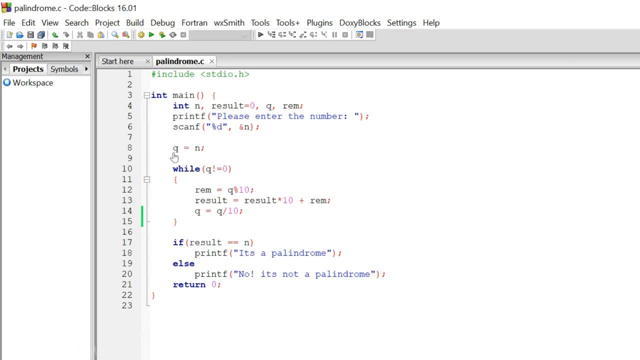 the input from the user. Then we put this inside the q variable and we put this whole logic inside the while loop. And here in this while loop we are checking the condition that q must not be equal to zero. Now, by checking this condition we can get outside of this loop. 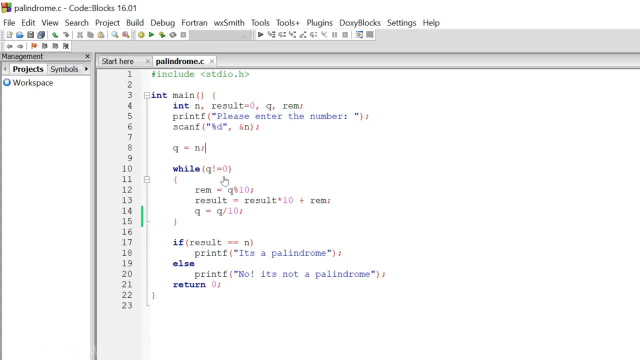 if q is equal to zero, That means our question is equal to zero. This simply means that after obtaining the last number of our reverse number, we should get outside of this loop and check if result is equal to n or not. If result is equal to n, 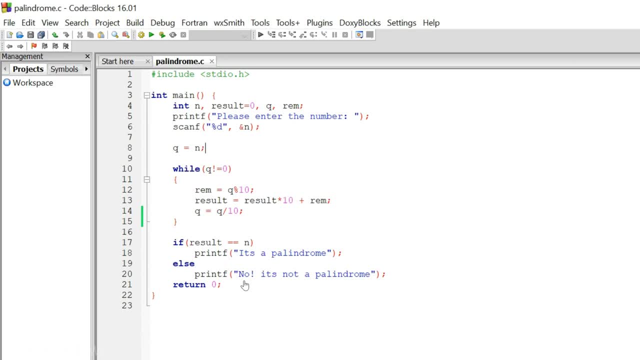 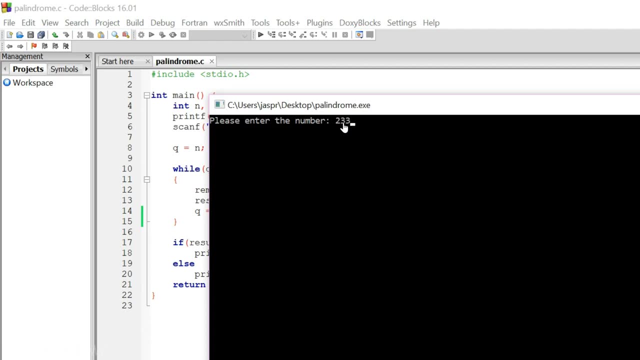 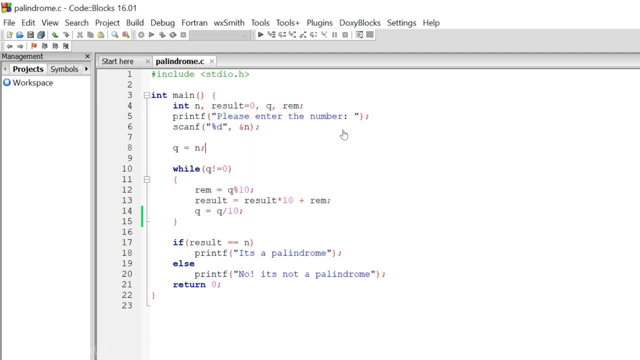 then we can simply say it is a palindrome. Otherwise we say: no, it is not a palindrome. Let's execute the code now. Here suppose I enter the number two, three, three, two and hit enter. It says it is a palindrome. Let's execute the code once again.